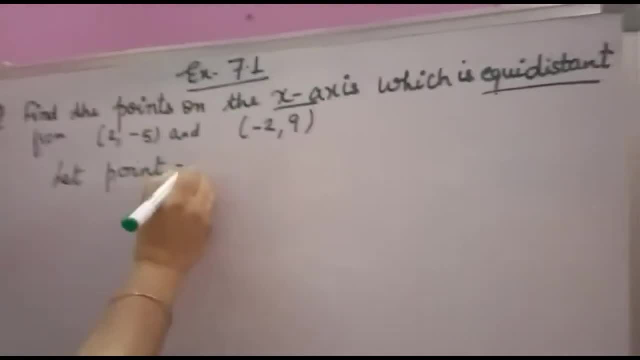 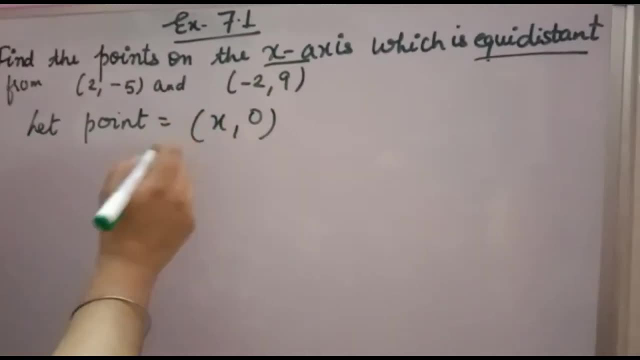 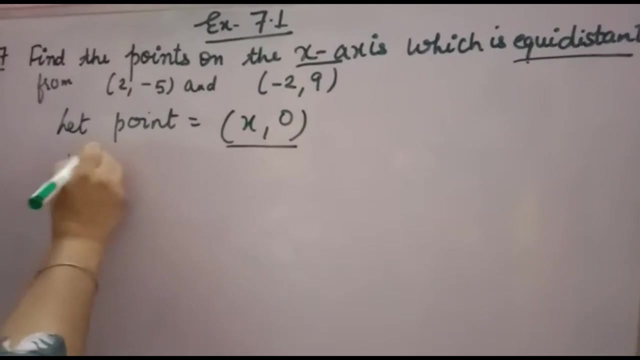 point is equal to x and 0. If suppose it is on y-axis, we will take 0 and y. If x-axis x and 0, you will take Now distance of this point from 2, minus 5.. So distance of x is 0 from. 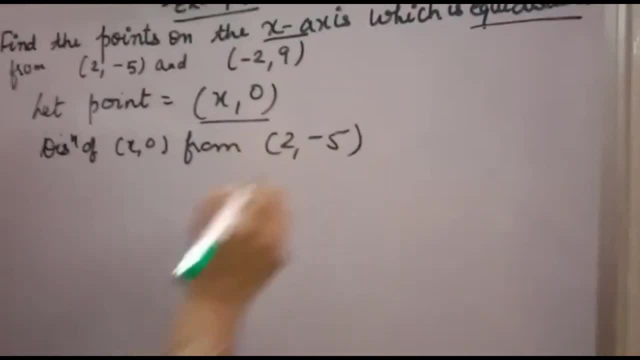 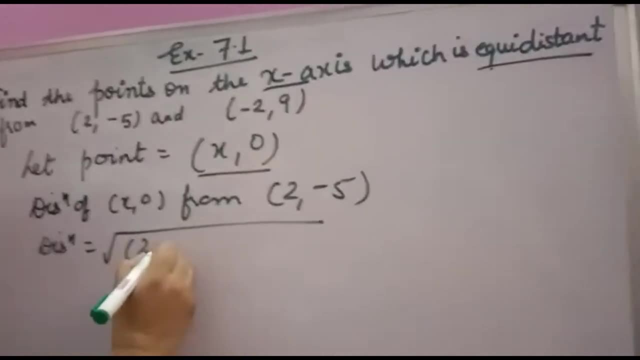 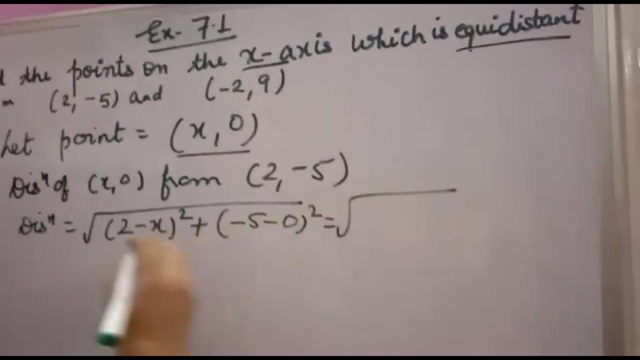 2, minus 5.. You will solve by distance formula. Distance will come. x2, minus x1 means 2, minus x, whole square plus y2, minus y1, that means minus 5, minus 0, whole square Now 2, minus x. 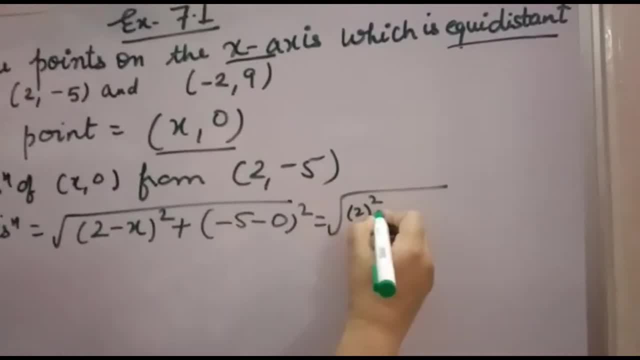 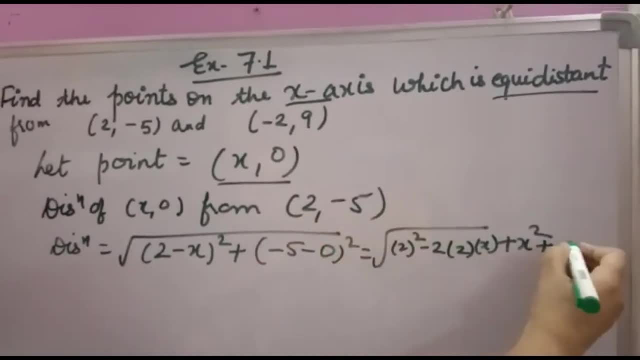 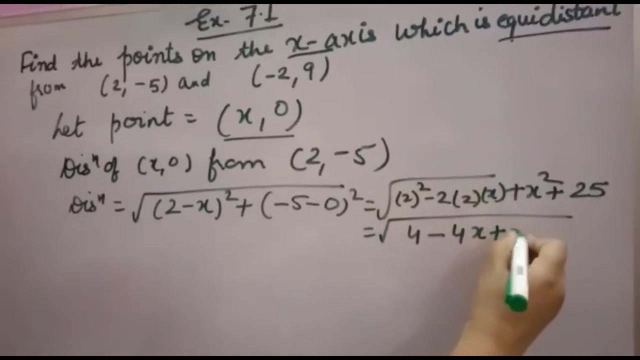 A minus b whole square, you will get 2 square minus 2 into a into b plus b square plus minus 5 square, you will get 25.. Now 2 square is 4, 2 into 2 into x, 4x plus x square plus 25.. Now 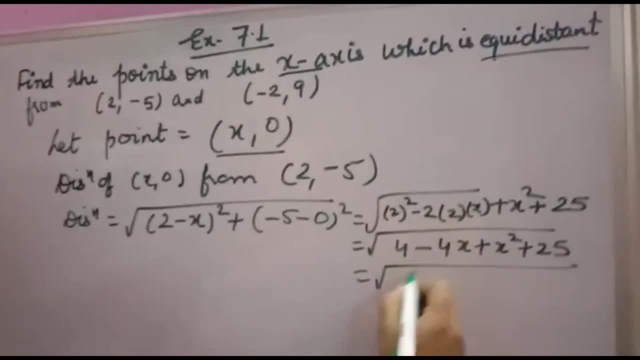 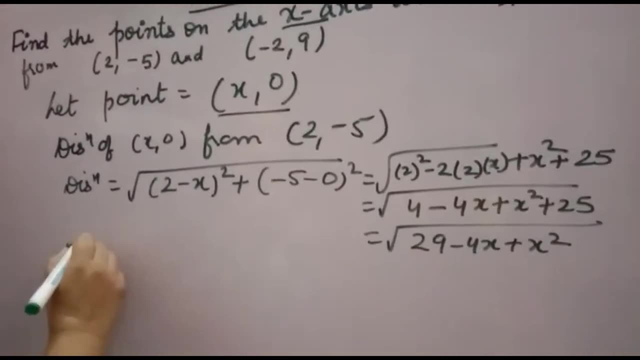 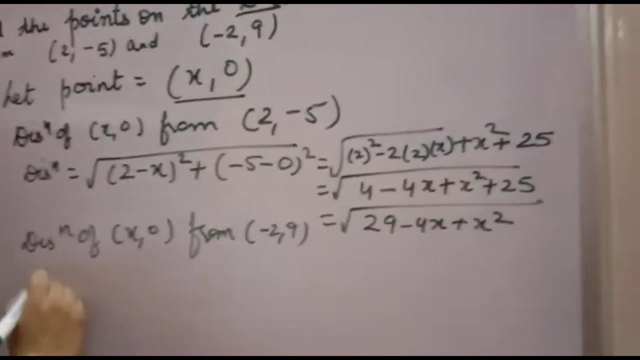 you will solve further. You will get 4 plus 25, 29 minus 4x plus x. square. Now distance of x is 0 from point minus 2, 9.. You will find by distance formula, Distance will come x2,. 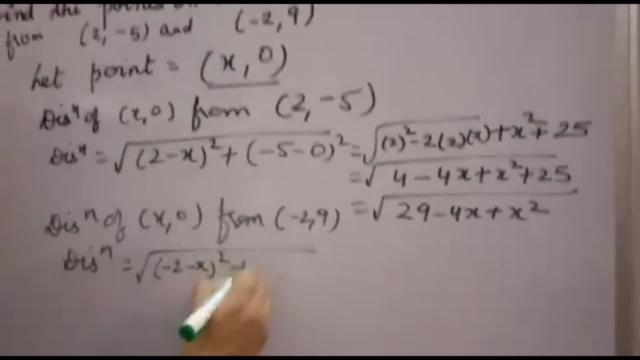 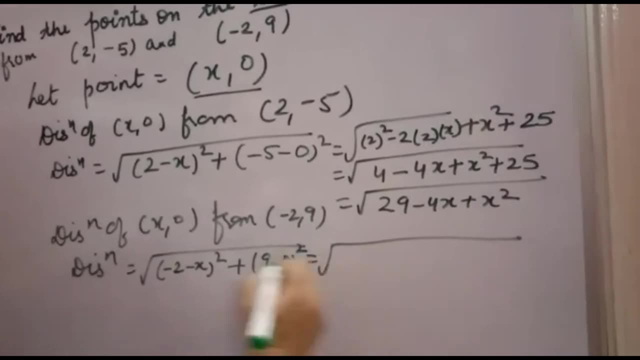 minus x1, minus 2, minus x whole square plus 9 minus 0 whole square, Now minus. you can take common, So you will get minus square is plus only, So you will get 2 plus x, whole square plus 9. 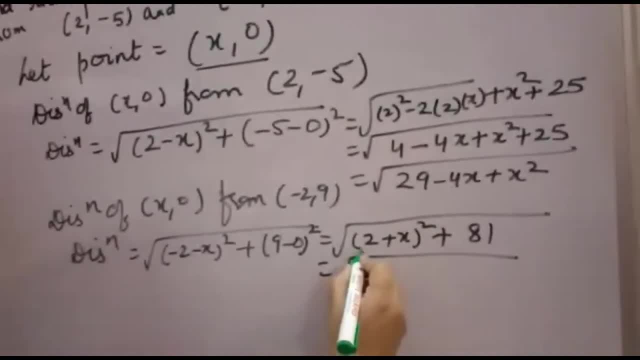 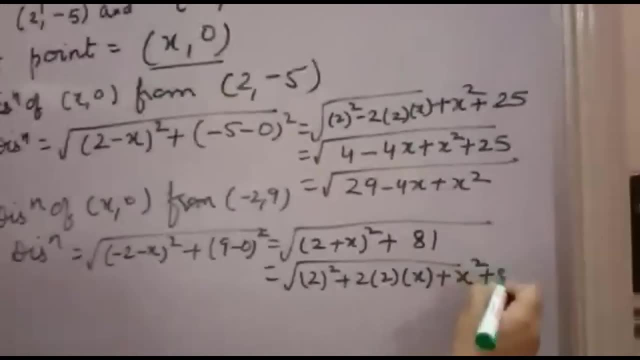 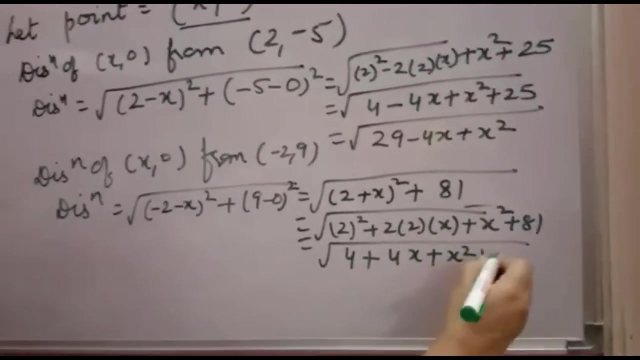 square is 81.. Now a plus b whole square you will open. you will get a square plus 2 into a into b plus b square plus 81. Now 2 square is 4, 2 into 2 into x is 4x plus x square plus 81.. Now 4 plus 81 is 85.. 85 plus 4x. 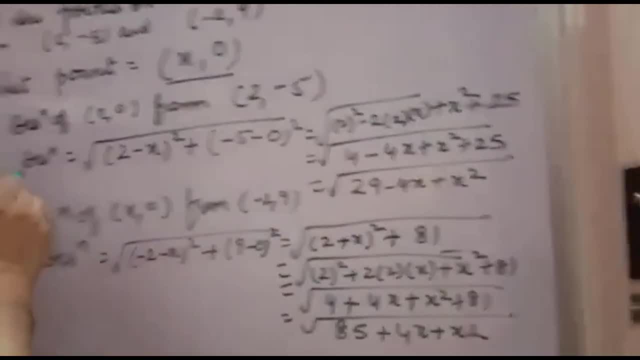 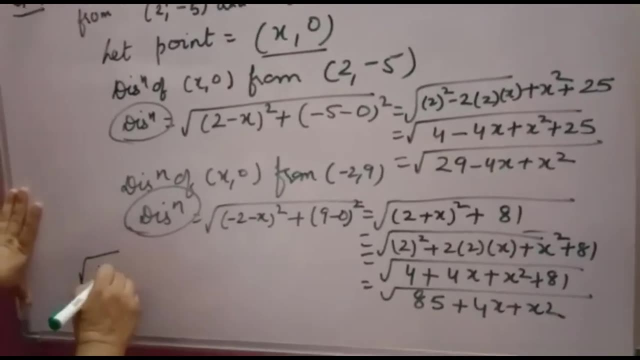 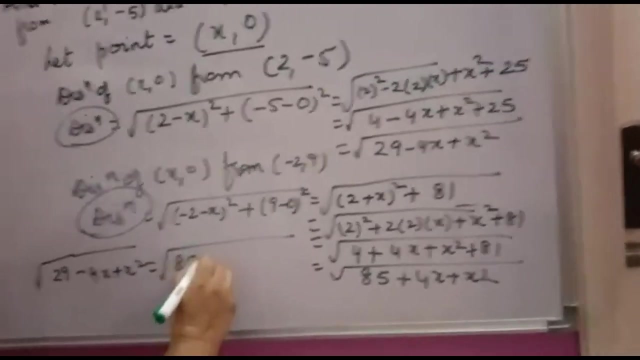 plus x square. So equidistant means this distance and this distance is same, So you will keep them equal. So root 29x minus 4x plus x square root is on full equal to root of 85 plus 4x plus x square. 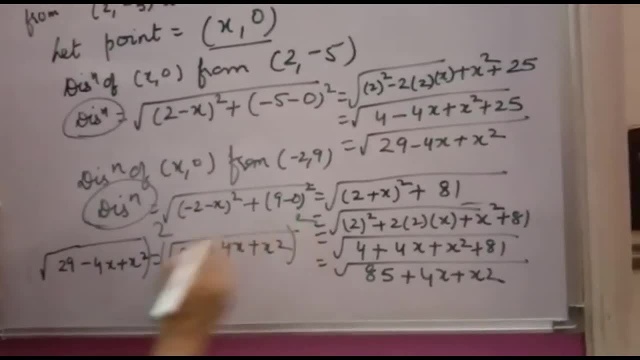 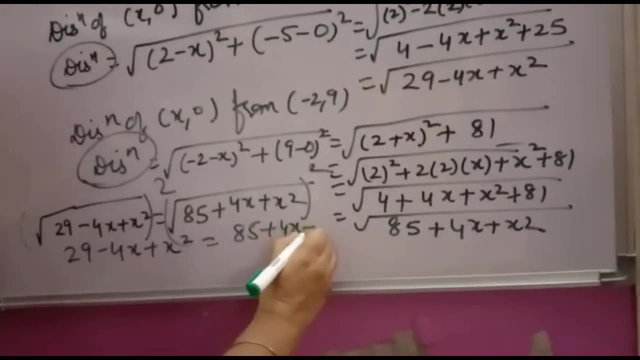 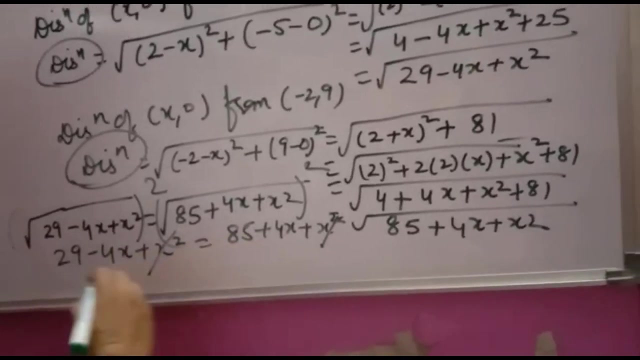 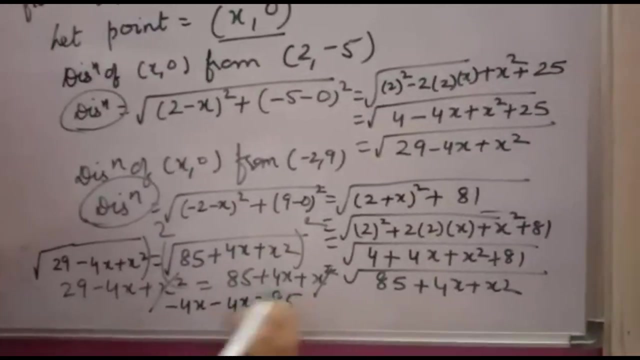 Now squaring both the sides. this root you can remove, you will get 29. minus 4x plus x square is equal to 85. plus 4x plus x square, Now x square, x square: cancel, because x square minus x square is 0.. Now minus 4x will remain here. this 4x you bring here, it will become minus 4x, 85.. This 29. 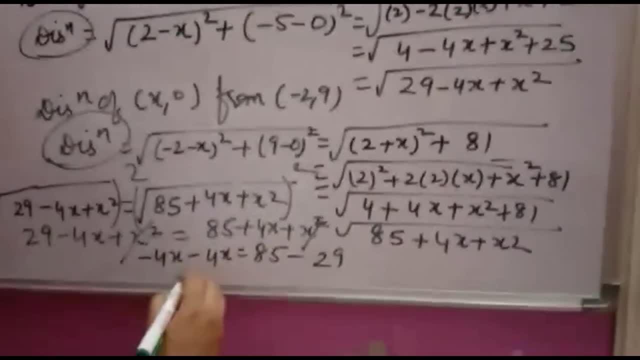 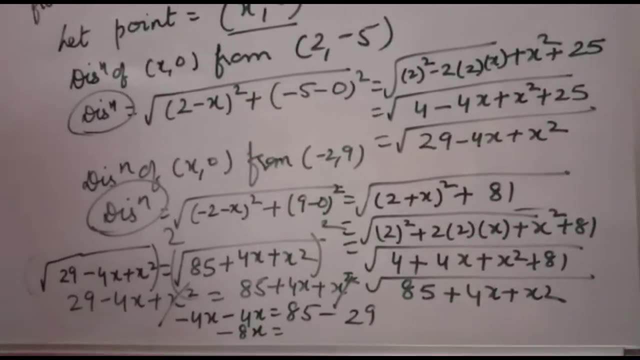 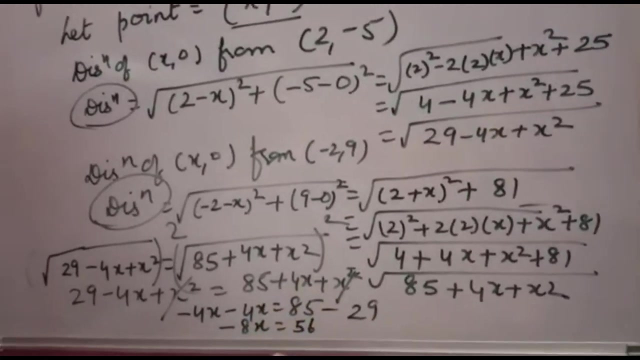 you will take that side and 85 you will write as it is minus 4x. minus 4x is minus 8x. Now, 85 minus 29, what will come? 85 minus 29, you will get 56. you will get 56 and plus because 85 is bigger. 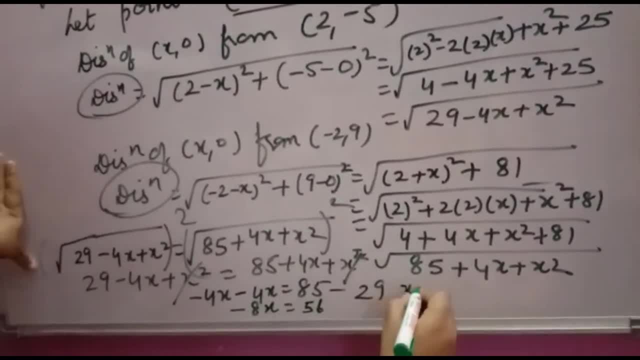 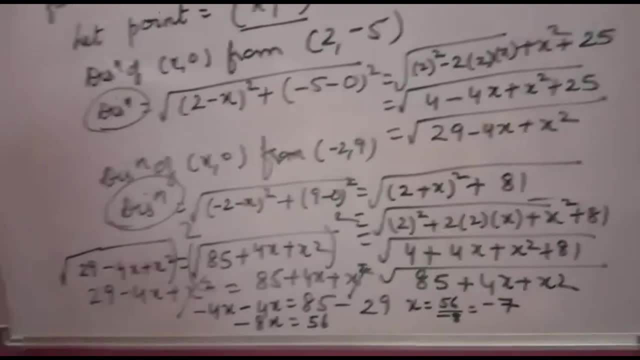 Now minus 8x, So x is equal to 56. So x will come 56 over minus 8, that is minus 7.. 8, 7 is a 56 and minus will come as it is. So required point will come which is equidistant from the given point is: 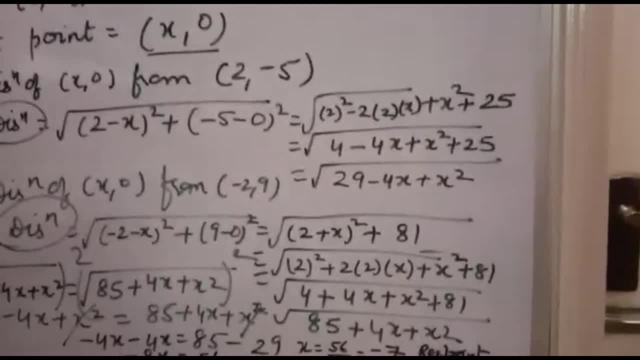 because you took x is 0, x came minus 7.. So minus 7: 0.. So minus 7: 0 is required, point. Thank you. 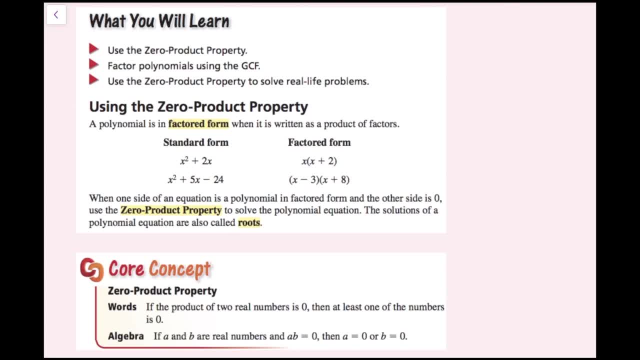 In this lesson, we're going to be using the zero product property, factoring polynomials, using the greatest common factor, and using the zero product property to solve real-life problems. A polynomial is in factored form when it is written as a product of factors.